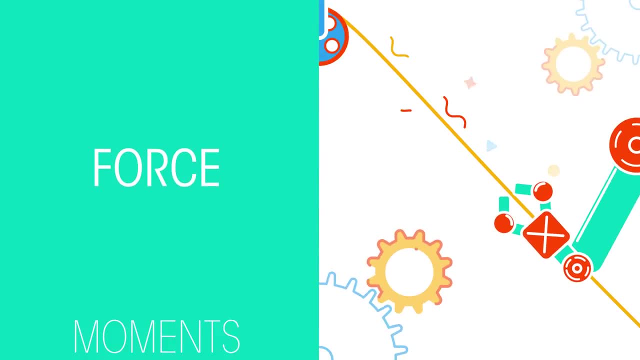 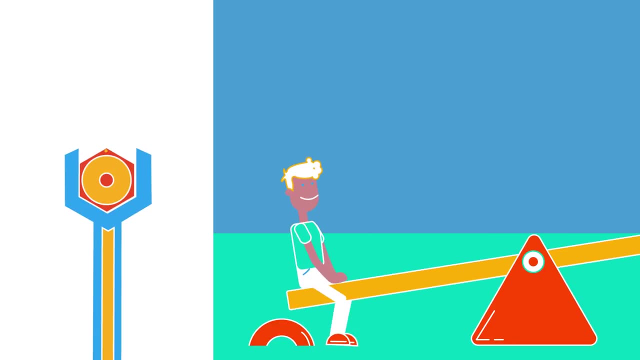 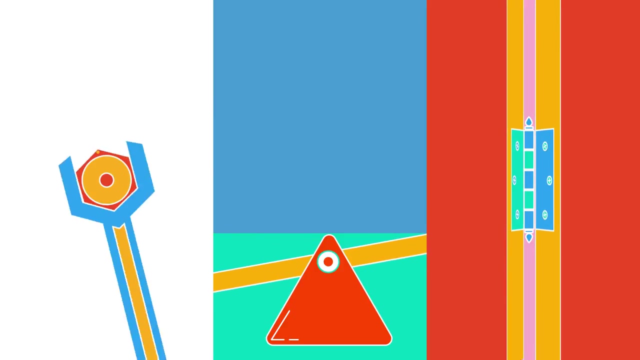 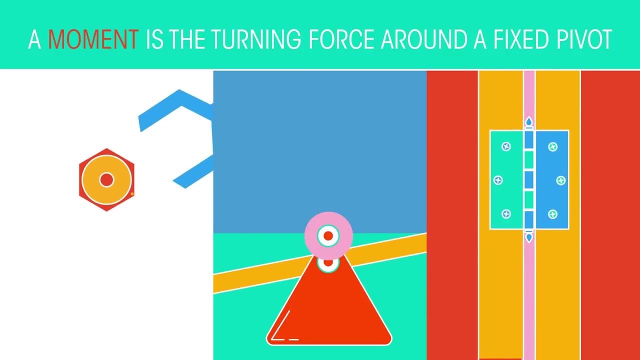 Think of a spanner loosening a fixed nut, or a child on a seesaw, or a door opening around a fixed hinge. All of these things are connected by something called moments. A moment is the turning force around a fixed pivot. The pivot is the nut or the middle of the seesaw or the hinge. 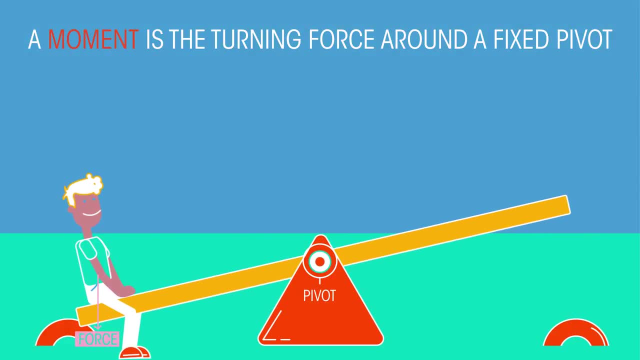 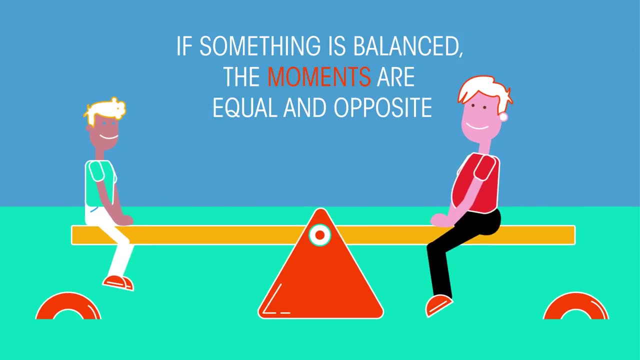 We can have one moment acting which results in a turning force, Or if something is balanced or in equilibrium. the moments are equal and opposite. To be balanced, this lighter child needs to sit further away from the pivot and the heavier child needs to be closer. This is because the size of a 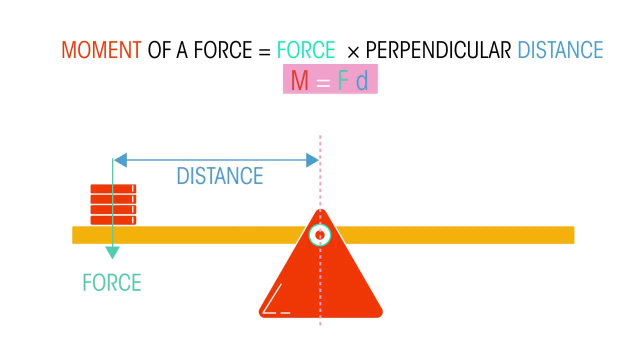 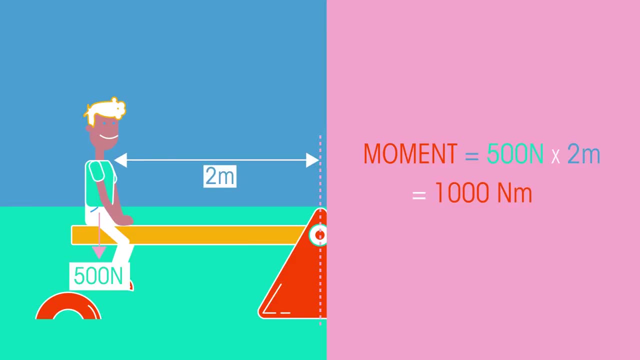 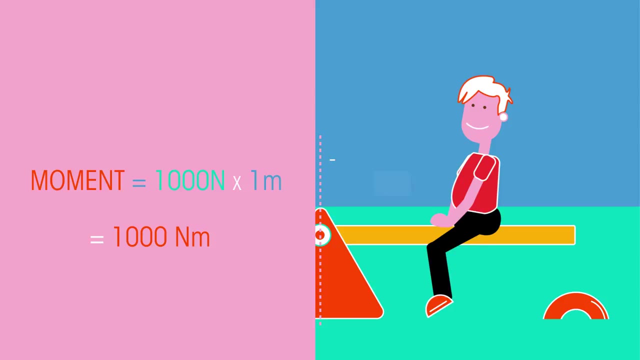 moment is determined by the force and a distance. So the moments of the lighter person is 500 Newtons multiplied by 2 meters, 1000 Newton meters, And the heavier person is a thousand times 1 meter. to also give 1000 Newton meters, They're perfectly balanced on their seesaw. 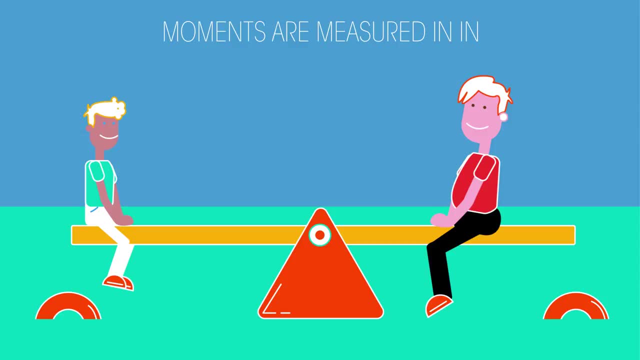 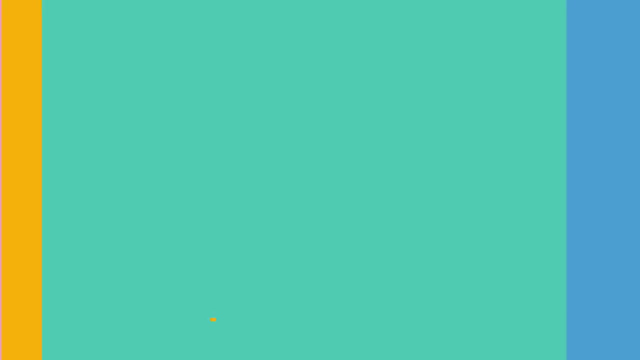 Did you notice that moments are measured in Newton meters NM, because force is measured in Newtons N and distance in meters. Note that the distance must be the perpendicular distance from the pivot to force. Here's another example. Can you work out what moments the woman is applying? 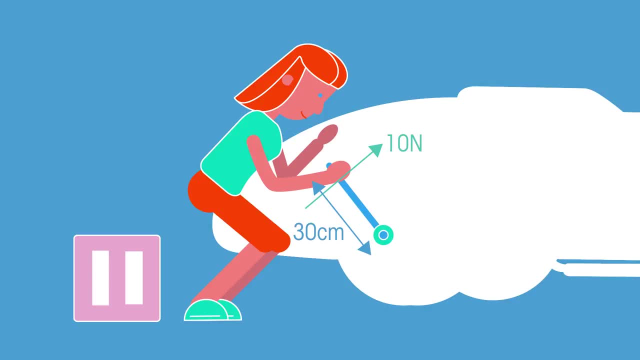 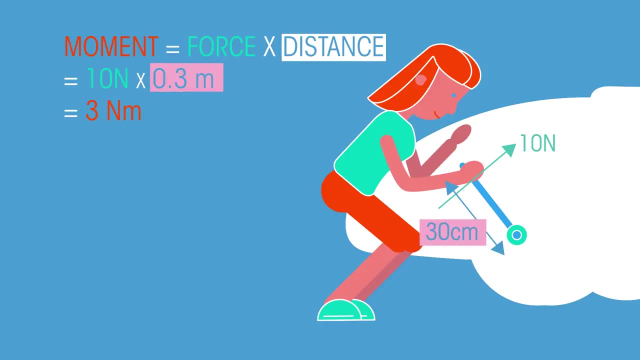 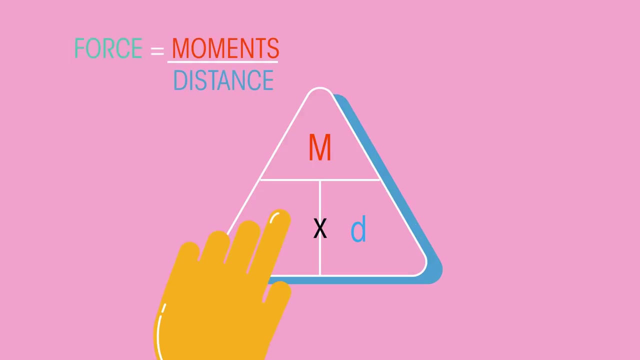 to tighten the wheel nut. Pause the video and work it out. Did you get 3 Newton meters? Were you careful to change the 30 centimeters into meters? We can also place this formula into a formula triangle: Force equals moments divided by distance. Distance. equals moments divided by force. 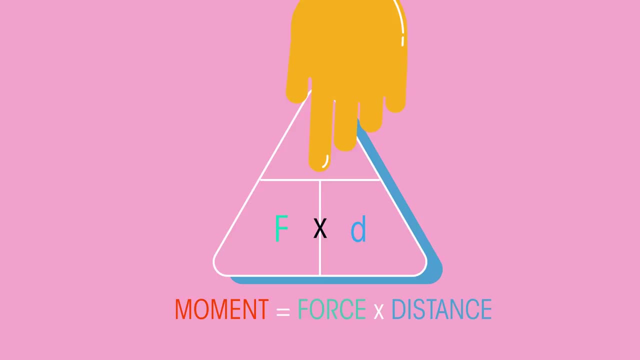 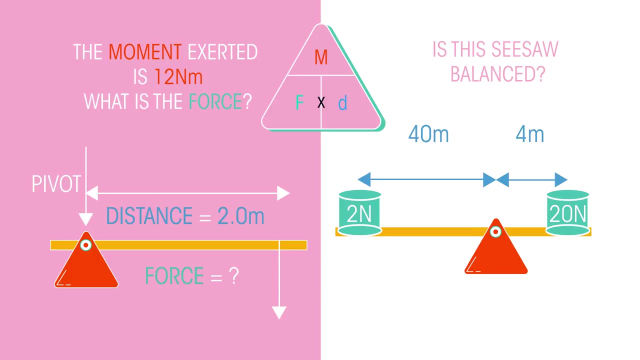 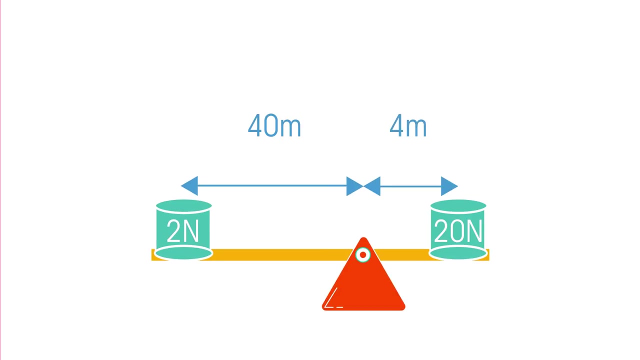 and moments and distance. The distance is the distance between the moments and the distance, as we already know, is force times distance. Here are two more questions for you, to try Pause the video and work them out. Did you get both questions right? For this, seesaw? we do actually say: 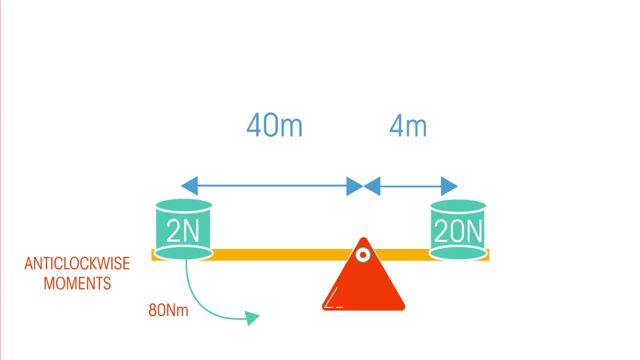 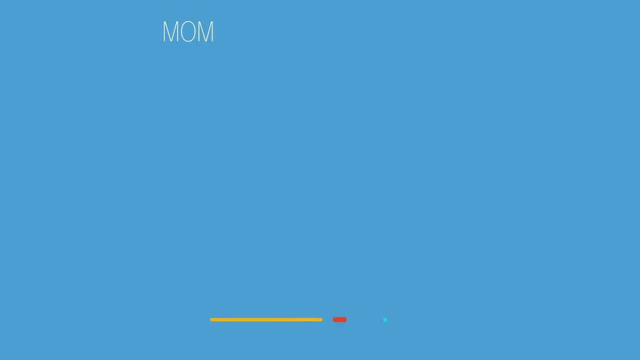 clockwise moments and anti-clockwise moments, And for something to be balanced, the clockwise and anti-clockwise moments must be equal. So there we have moments. They're measured in Newton meters and are the force multiplied by the perpendicular distance.